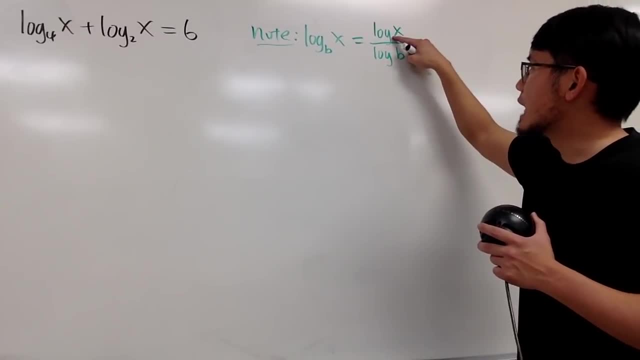 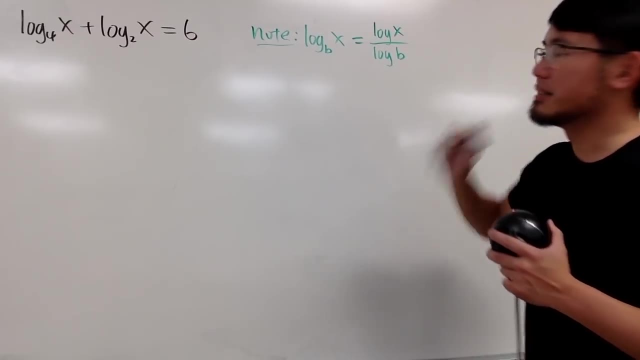 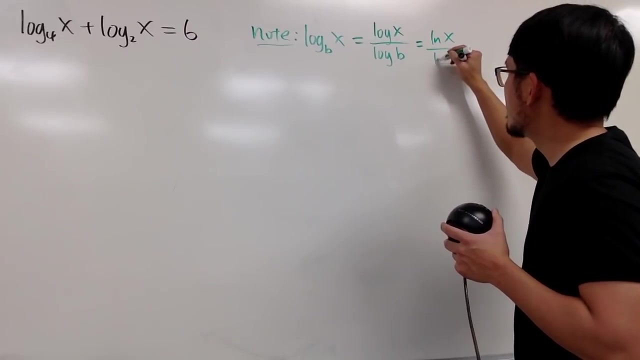 which is b. Notice that as long as the top and bottom they have the same log, you're okay. This is technically log base 10,, log base 10.. And of course we like to use the natural log. so in fact this is the same as saying natural log of x over natural log of b. 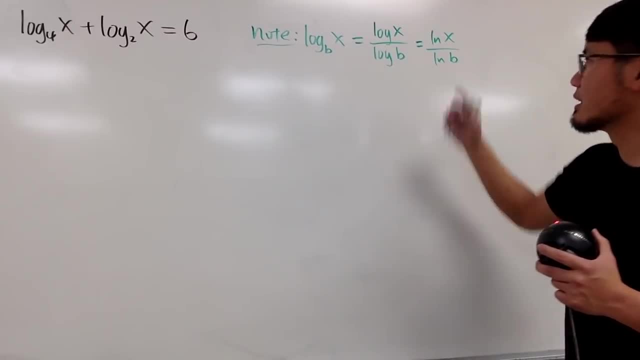 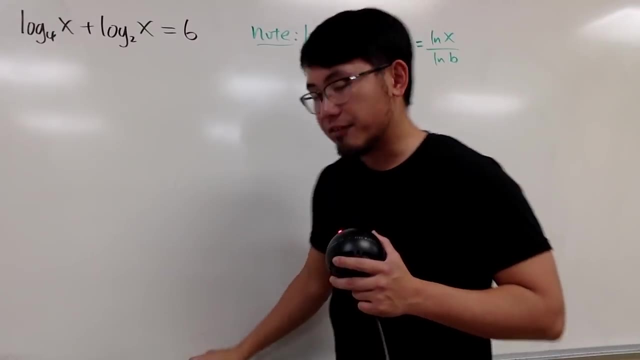 And natural log is of course log base e, and then on the bottom here we have log base e And again you can put whatever number that you want right here. but I'll stop right here. So that's the first change that we need to do. 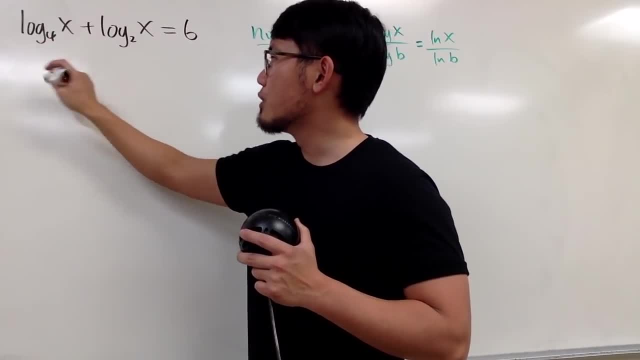 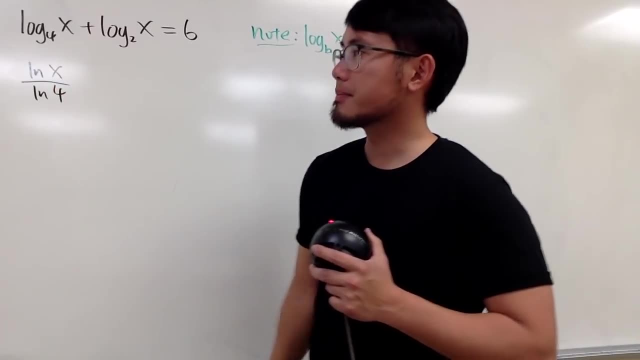 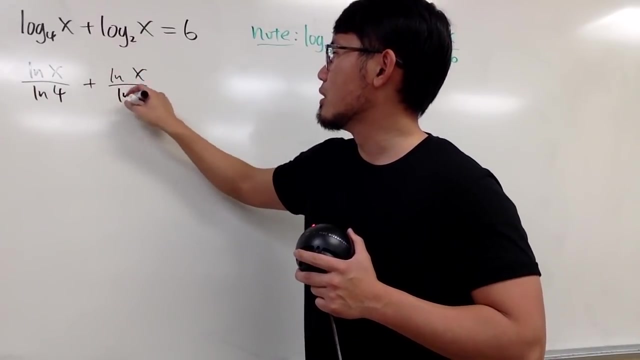 Let's look at this right here: The base is 4.. This means I will just take natural log and then we'll put the x right here over I'll put down natural log of 4, like that, And then for this right here let's just add natural log of x over natural log of 2, this time equals 6.. 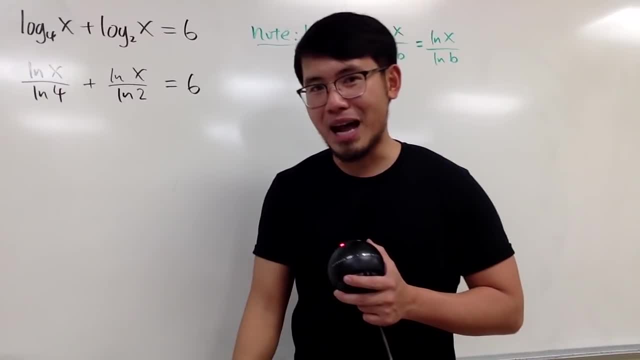 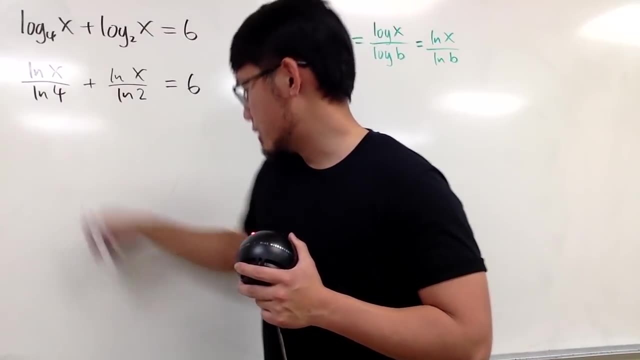 Good. So that's pretty much the first. And now look at 4. right here, 4 is the same as 2 squared. Why do we need that? Because let's just put this down in green, so we have some Christmas color. 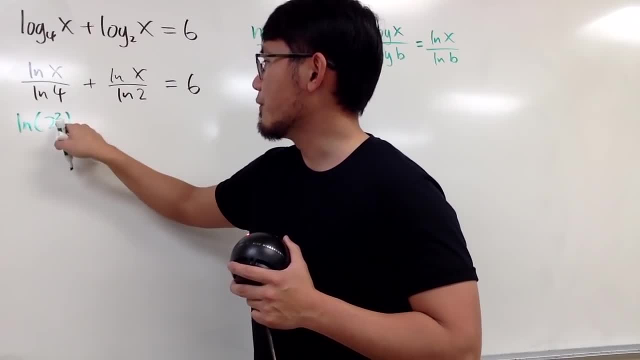 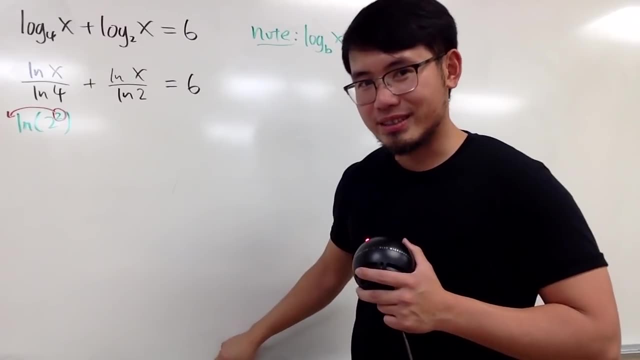 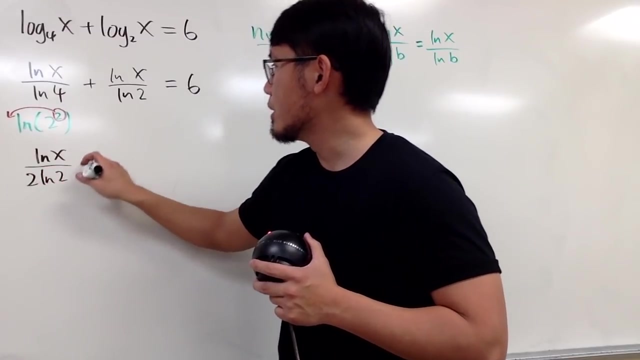 Natural log of 2 squared right for the 4, because when we have 2 squared we get to bring the power 2 to the front for that. So you see, this equation becomes natural log of x over 2, natural log of 2,. 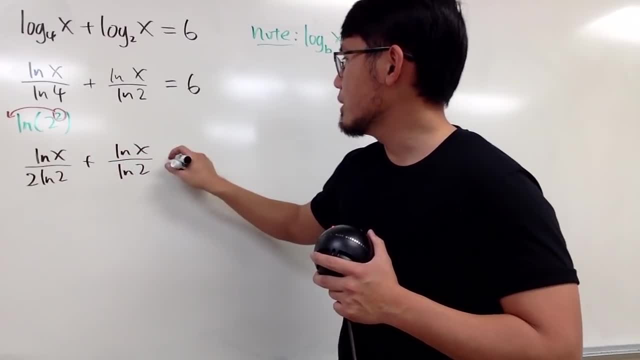 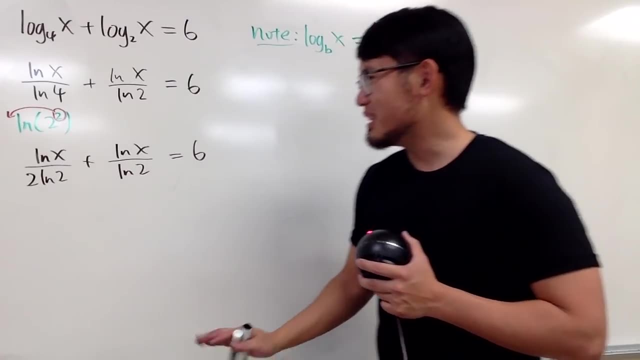 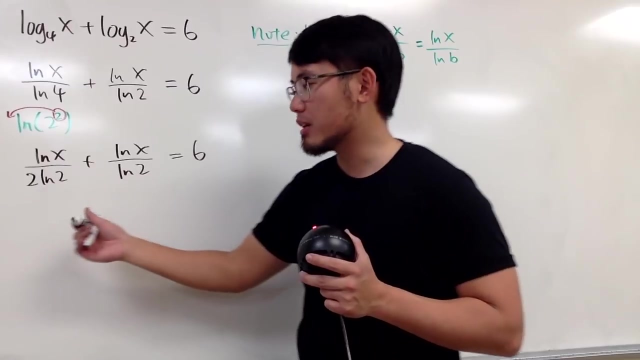 natural log of x over natural log of 2, equals 6.. So we are lucky. they both have the natural log of 2 in common. So this is much more doable. And to finish this up, let's just multiply everybody by the lowest common denominator, namely 2 log. well, 2 natural log of 2, like this: 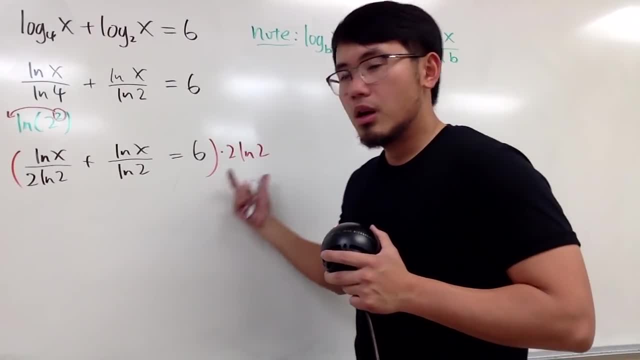 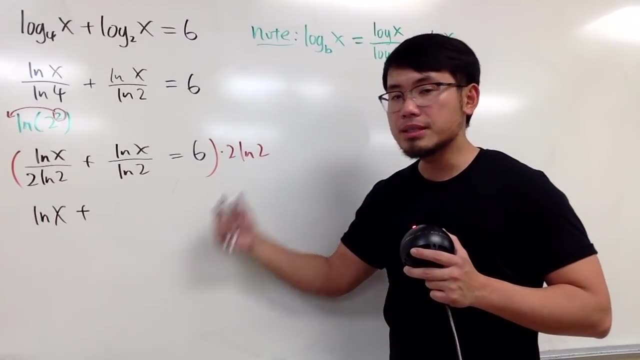 So let's multiply by 2, natural log of 2.. Okay, when we multiply this and that, of course they cancel and we just get natural log of x And we add. when we do, this times that natural log of 2 cancel. 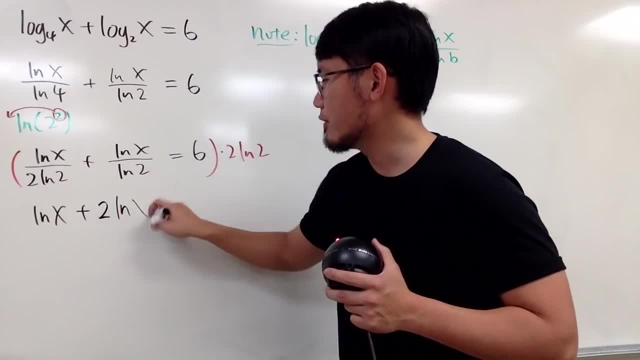 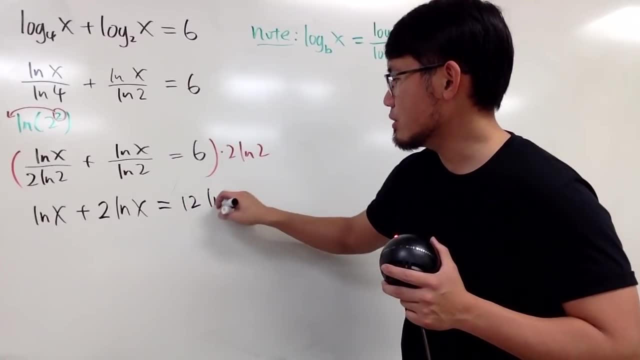 We have 2 times this. so I put down 2, natural log of x and this is equal to, and. when we do this, times that 6 times 2 is 12, and then we have the natural log of 2, like this: 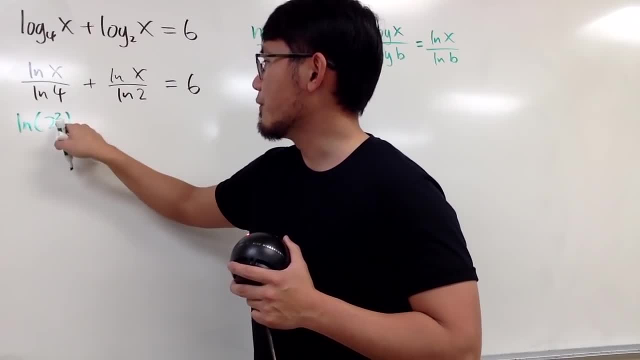 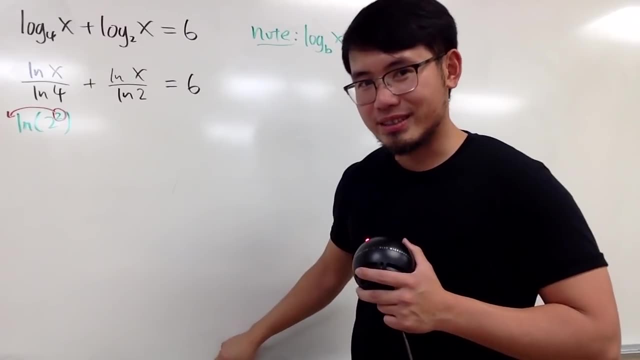 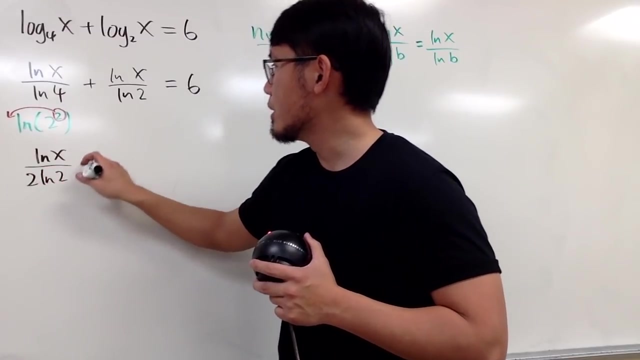 Natural log of 2 squared right for the 4, because when we have 2 squared we get to bring the power 2 to the front for that. So you see, this equation becomes natural log of x over 2, natural log of 2,. 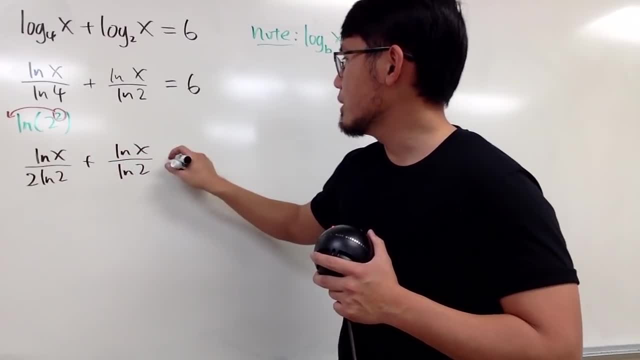 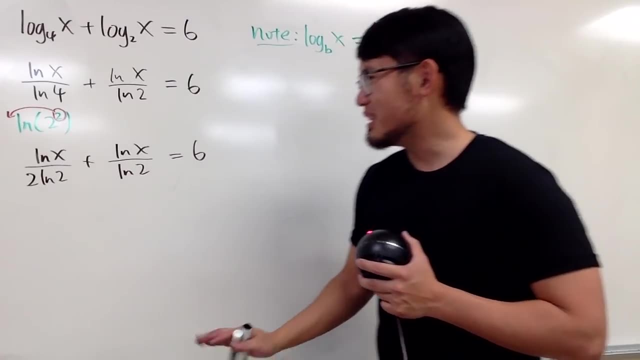 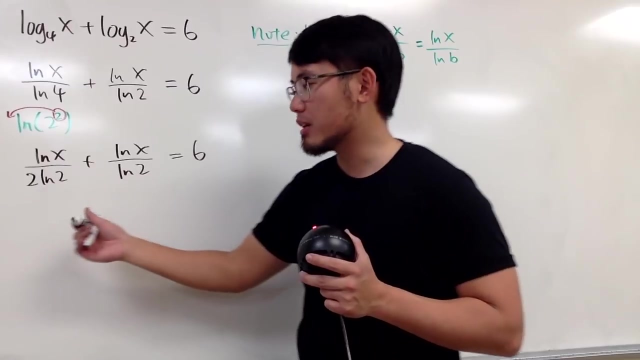 natural log of x over natural log of 2, equals 6.. So we are lucky. they both have the natural log of 2 in common. So this is much more doable. And to finish this up, let's just multiply everybody by the lowest common denominator, namely 2 log. well, 2 natural log of 2, like this: 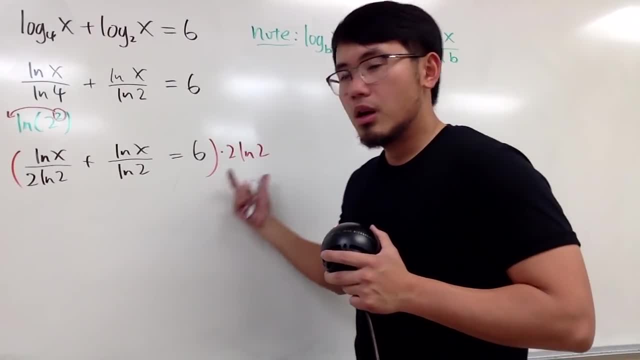 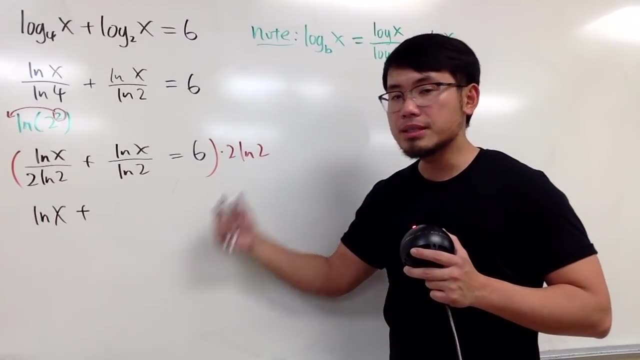 So let's multiply by 2, natural log of 2.. Okay, when we multiply this and that, of course they cancel and we just get natural log of x And we add. when we do, this times that natural log of 2 cancel. 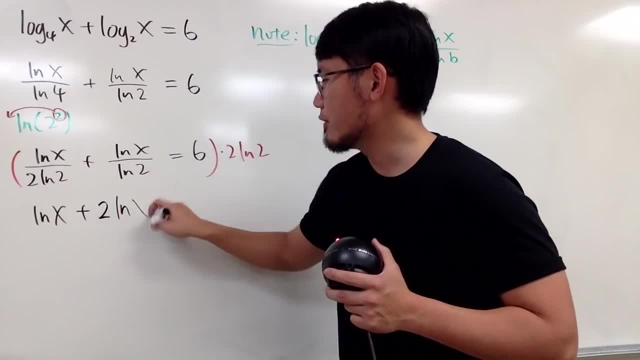 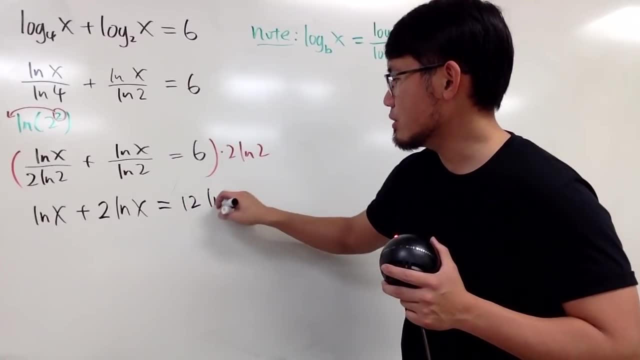 We have 2 times this. so I put down 2, natural log of x and this is equal to, and. when we do this, times that 6 times 2 is 12, and then we have the natural log of 2, like this: 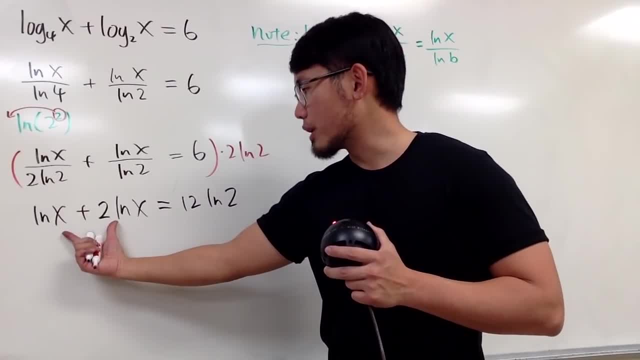 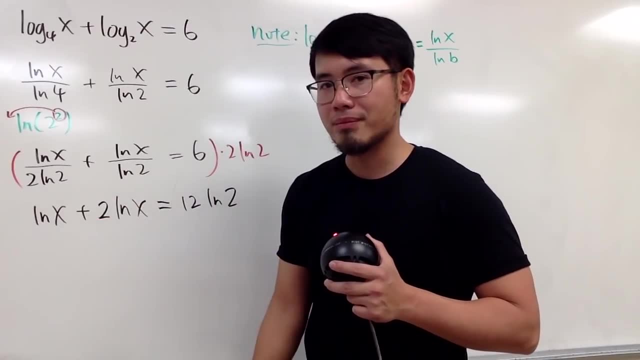 And now for this equation, for this part right here of the equation, I want to combine the logarithms, And to do so you have to make sure the coefficients are 1.. This is now 1. But it's okay, because we can bring this and make it into a power. 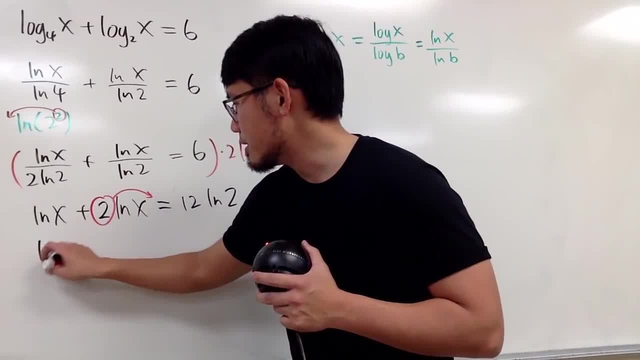 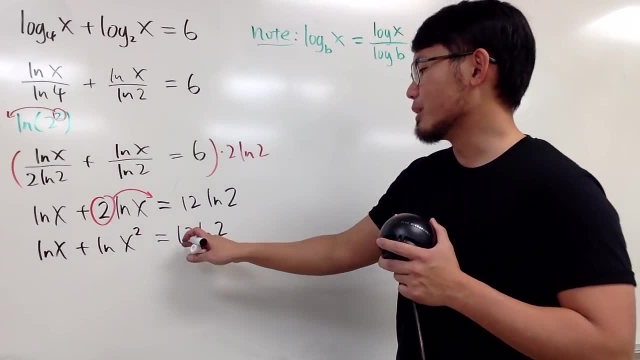 So it's like the backwards of that. So when we do that, this is this natural log of x plus natural log of x squared, and this is 12 natural log of 2.. Of course, you can bring the 12 up and perhaps let's do that. 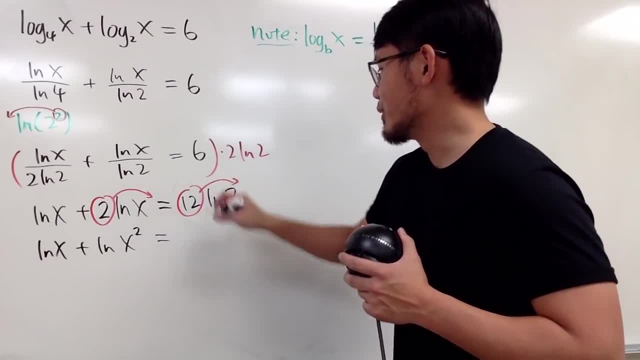 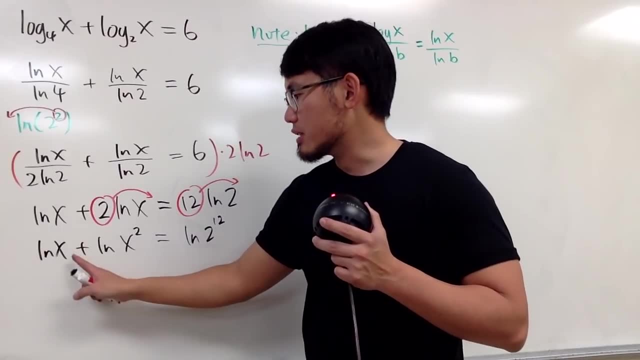 Why not? You guys will see, this is actually going to be pretty cool. Natural log of 2 to the 12th power. Anyway, this right here is what The sum of two natural logs is: The natural log of the product of this and that. 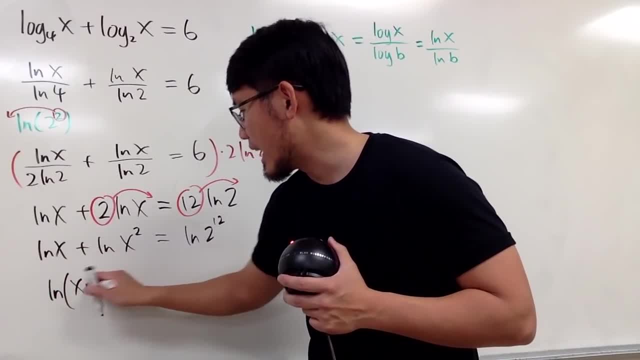 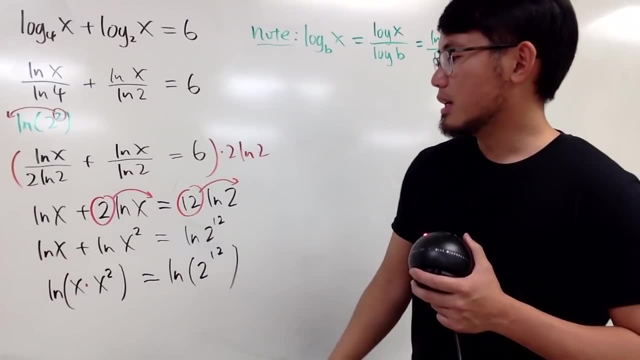 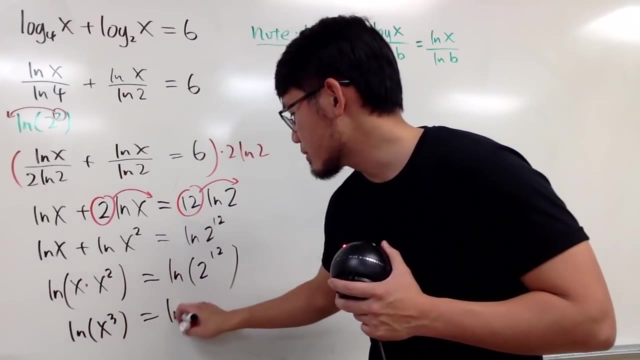 In other words, this is natural log of x times x squared, and this is natural log of 2 to the 12th power, like this: And now, of course, this is natural log of x to the 3rd power and this is natural log of 2 to the 12th power. 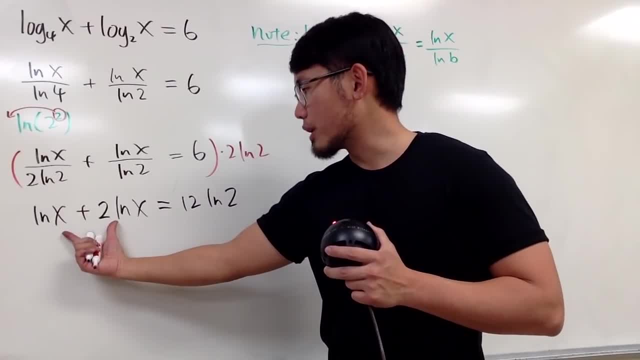 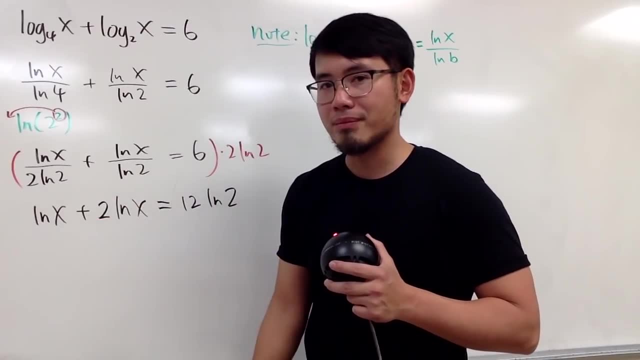 And now for this equation, for this part right here of the equation, I want to combine the logarithms, And to do so you have to make sure the coefficients are 1.. This is now 1. But it's okay, because we can bring this and make it into a power. 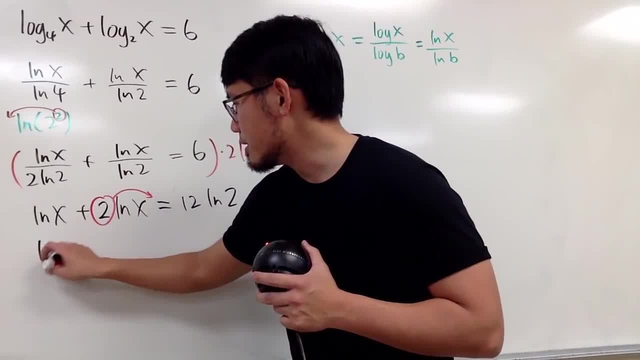 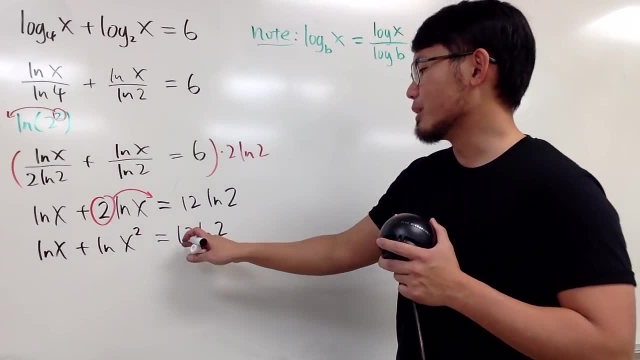 So it's like the backwards of that. So when we do that, this is this natural log of x plus natural log of x squared, and this is 12 natural log of 2.. Of course, you can bring the 12 up and perhaps let's do that. 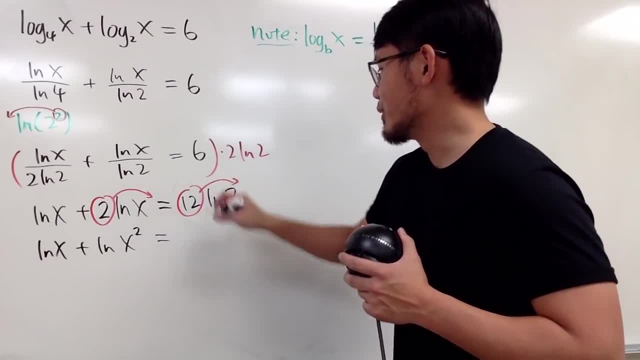 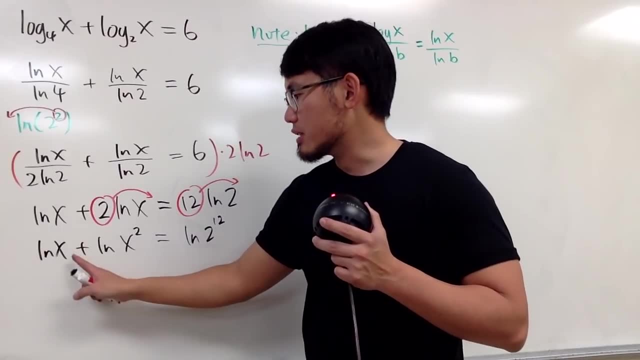 Why not? You guys will see, this is actually going to be pretty cool. Natural log of 2 to the 12th power. Anyway, this right here is what The sum of two natural logs is: The natural log of the product of this and that. 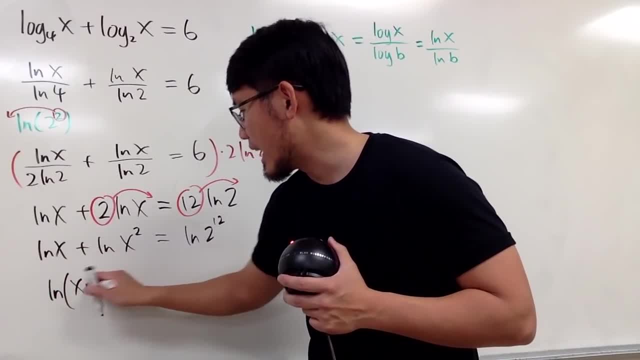 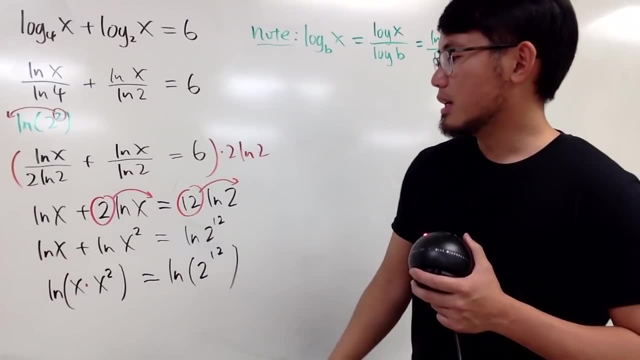 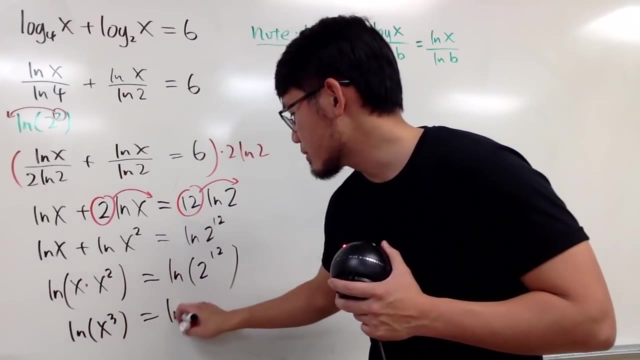 In other words, this is natural log of x times x squared, and this is natural log of 2 to the 12th power, like this: And now, of course, this is natural log of x to the 3rd power and this is natural log of 2 to the 12th power. 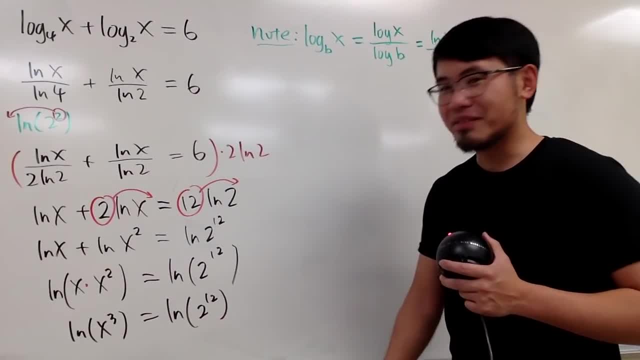 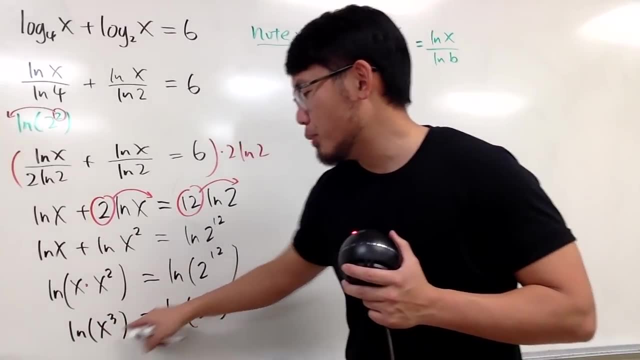 So this is pretty much a simplification that we have done so far And now check this out. So in the real world, when you have natural log equal to each other, that means the input have to equal to each other as well, because natural log is a one-to-one function. 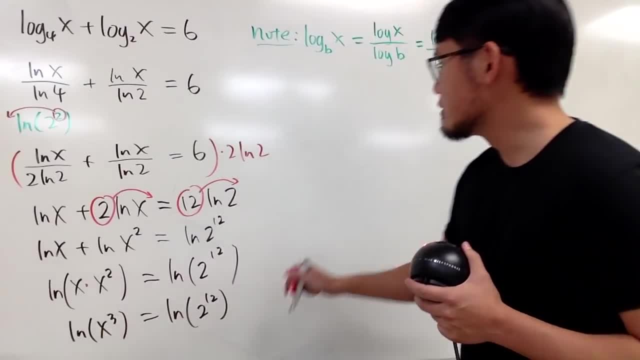 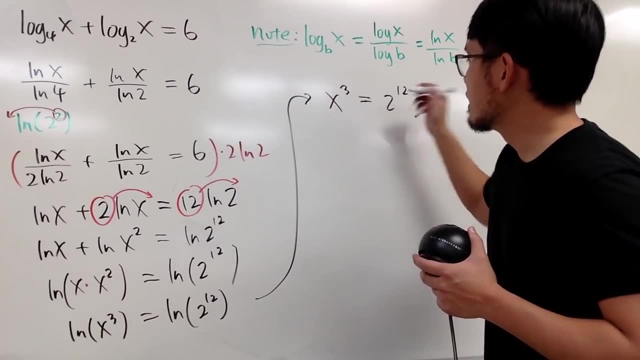 Therefore, we have: x to the 3rd power has to be the same as 2 to the 12th power, like that. And another way to look at this is, of course, you can do e to this power, e to that power. but I think that explanation was better. 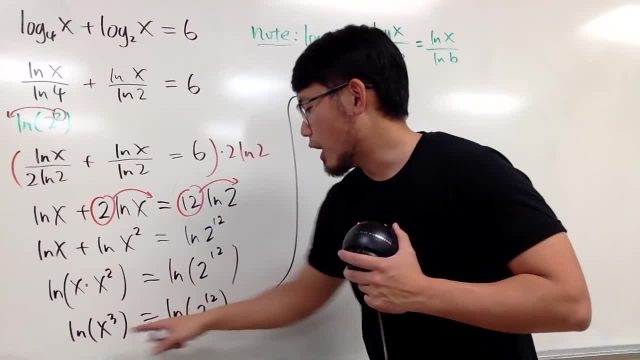 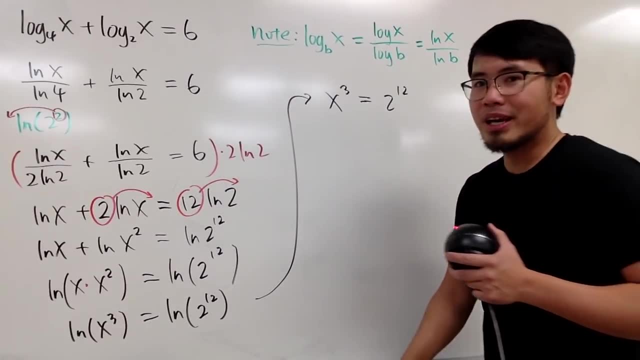 Natural log is a one-to-one function, meaning that If the output are the same, that means the input have to be the same. So we can draw this conclusion and you can just now take the cube root to both sides or maybe raise both sides to the 1- 3rd power. 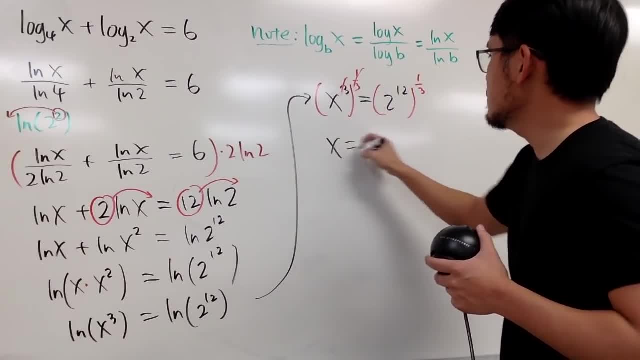 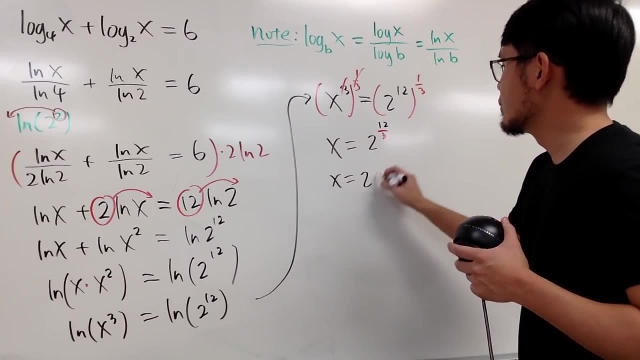 Perhaps this is more legit, so that this end up cancel and you get: x is equal to 2, and then this is 12 times 1, let's put this down, why not? which is x equals 2 to the 4th power, which is 16..